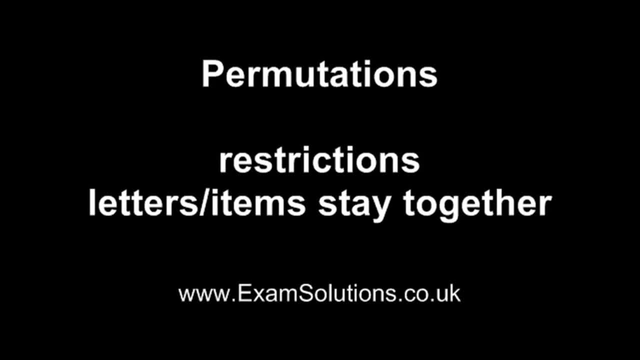 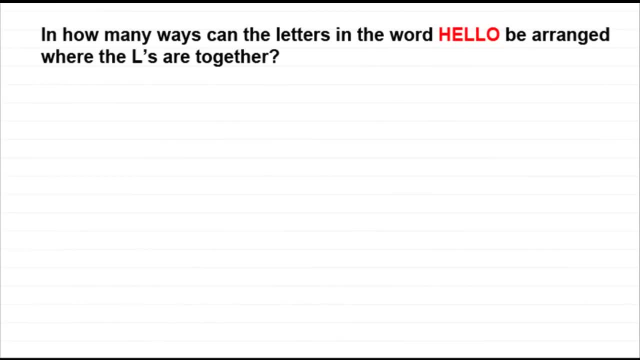 Hi, welcome to this, my fourth tutorial in the series: Permutations and Combinations. In this tutorial, what we're going to look at is how many ways we can arrange letters or items. where we're restricting the arrangements? We're restricting it to where letters or items stay together. 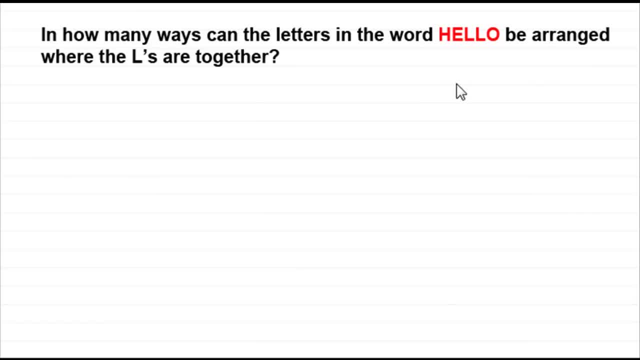 We've got this first example here. In how many ways can the letters in the word hello be arranged where the L's are together? Now, to do this, what I would encourage you to do is just write out the letters of the word hello. so we'll just do that, And what we do is we parcel the letters or items that have got. 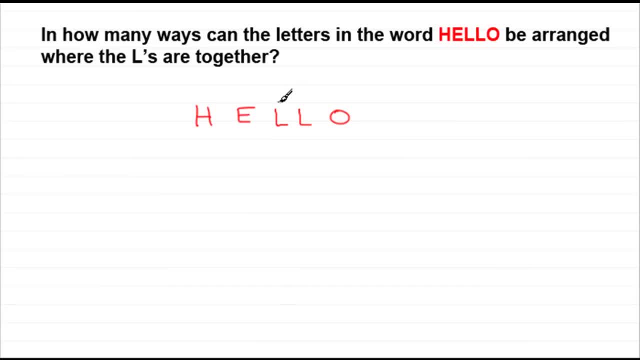 to stay together, And in this case it's the two L's, So we'll just put a circle round that. So, when we look at the number of arrangements, all we need to do is think of this as one, two, three, four letters. 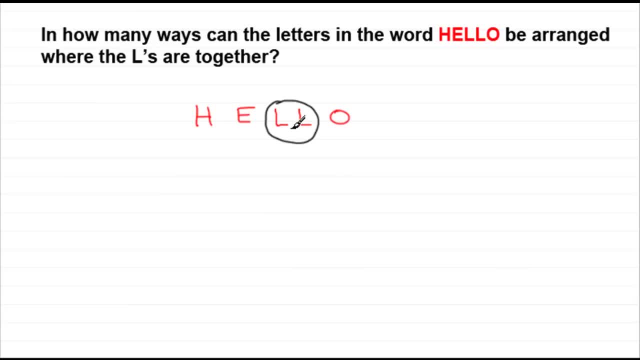 Okay, Think of this as four different items. So, when it comes to the number of arrangements, how many different ways can we arrange four different items? Well, we've discussed this earlier in tutorials. It's got to be four factorial. Four factorial, which we know is four by three, by two, by one, And if you work that out, you get that it equals 24.. 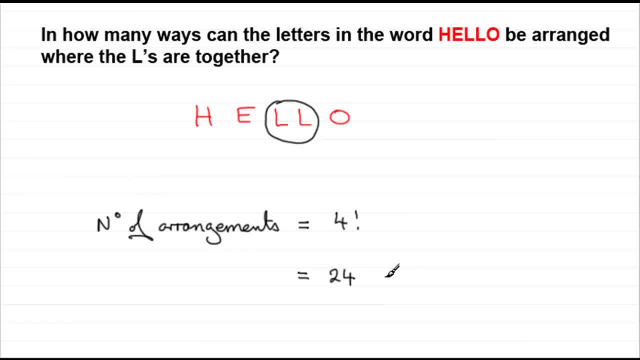 Okay, Well, that's fairly straightforward. But in my next example we take this to a slightly higher level. Okay Well, that's fairly straightforward. But in my next example we take this to a slightly higher level. Okay, Well, that's fairly straightforward. 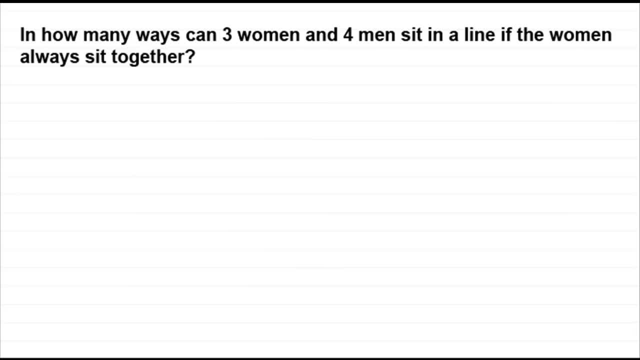 Okay, Well, that's fairly straightforward Now in this example. what we've got, then, is: how many ways can three women and four men sit in a line if the women always sit together? Well, for something like this, I tend to write, say, three women down, like this, but to identify that they're. 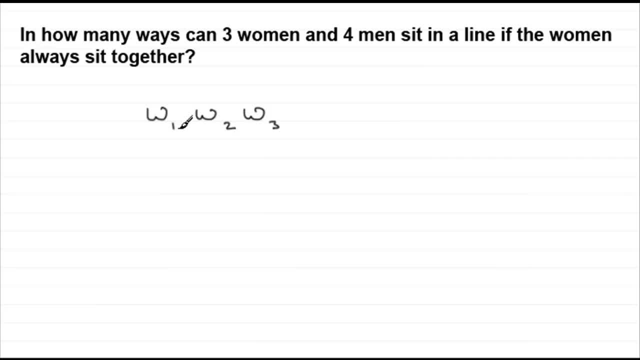 different. I just put some subscripts like this: this, two and three And the same for the men. We'll just have our four men and we'll label them one, two, three and four. Then we need to circle the women because they've got to sit. 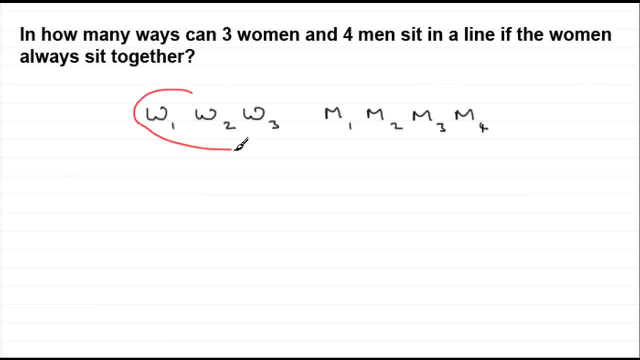 together. So we'll just stick a circle out here, And then, when it comes to working out the number of arrangements, we'll just put that intro in. I've got to think of how many different items have I got. Well, we've got one here, two, three, four, five. So we've 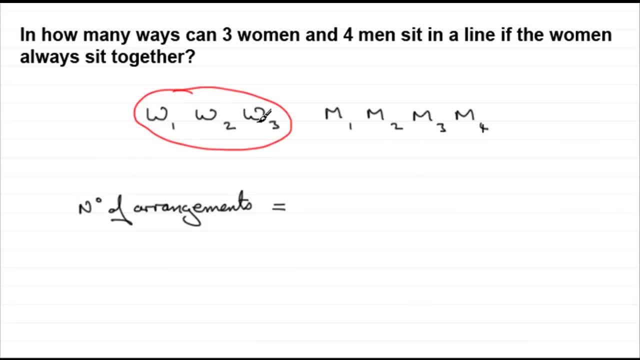 got five different items to arrange, So they can be arranged amongst themselves five factorial ways. So we'll just put that down as five factorial. However, unlike the first example inside this circle we've got three different items. So in any one of these five factorial arrangements these three items can rearrange themselves. 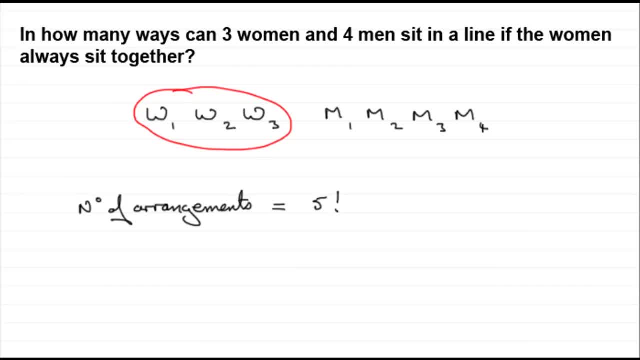 amongst themselves in three factorial ways. So what we've got to do is multiply this by three factorial: The number of items. The number of items. The number of items: The number of ways, then, that the women can rearrange themselves amongst themselves. 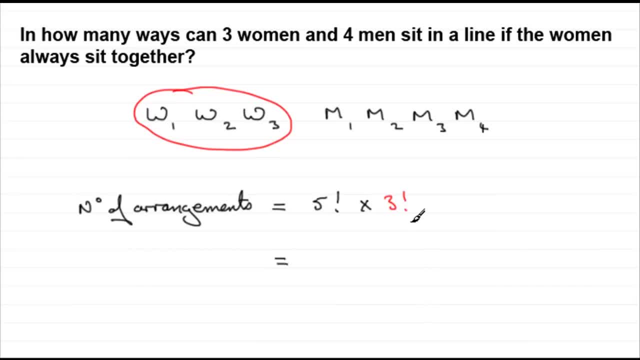 Well, if you work this out on your calculator, what you get is 720.. Okay, well, I hope you've got that one. Now, in my next example- the last example again, we extend this idea and go back to looking at arrangements of letters. 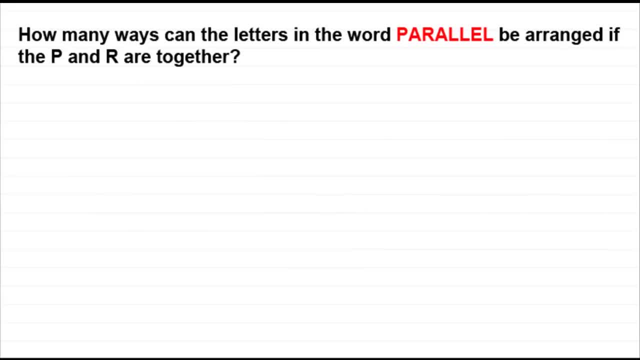 Now in this example, then what we've got is: how many ways can the letters in the word parallel be arranged if the P and the R are to stay together? Well, with this one? what I'd want to do is first of all write down these letters for the word parallel. So we're 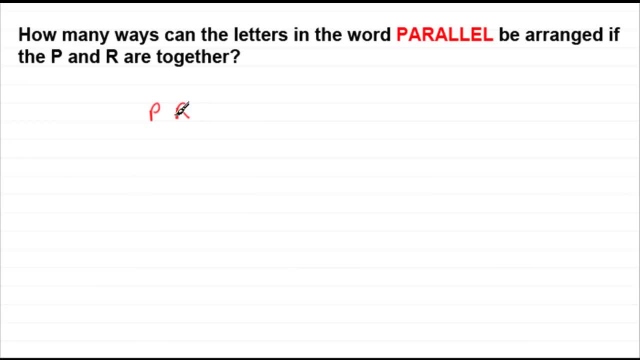 going to write P and an R. Okay, and I've purposely put these together now. So I'm going to write P and an R. We've got two A's- let's just write those down- and we've got three L's and an E. Now we've got to keep the P and the R together, And what I'm going to? 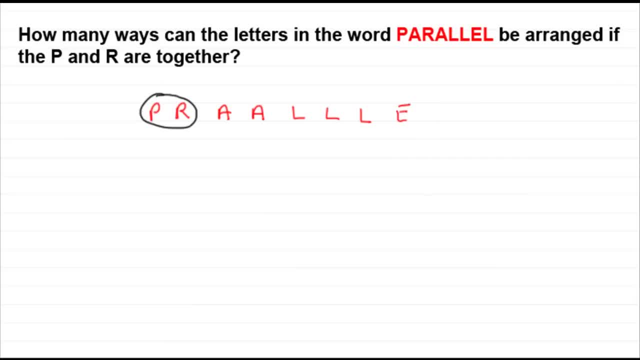 do is treat these letters as if they're all different. And to do that, what I need to do is look at the A's, for instance, and instead of having the two A's looking the same, just put some subscripts: A1, A2.. And when it comes to the L's, do exactly the same: L1, L2 and L3.. Now, if we're 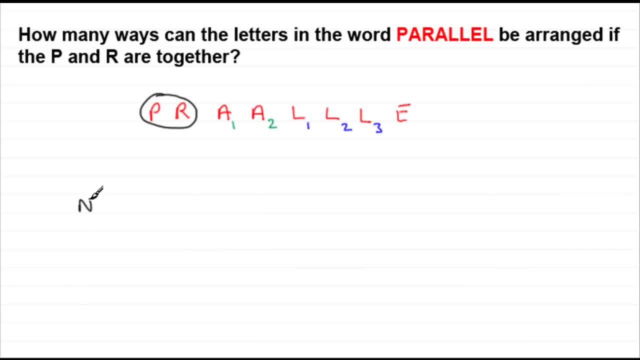 looking, then, at the number of arrangements, how many are they going to be? Well, first of all, if all the letters are treated as being different, we've got essentially one here: A3, A4, A6, A7.. Two, three, four, five, six, seven, Seven different letters, And those 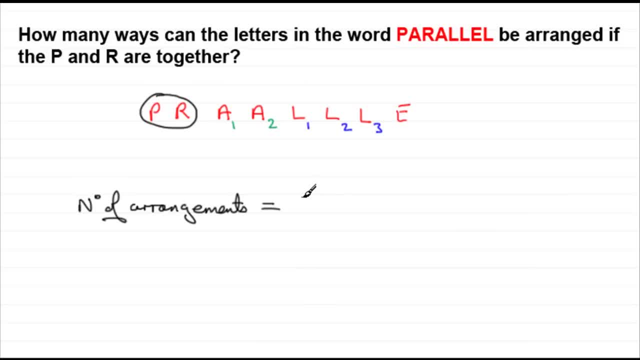 seven different letters can be rearranged amongst themselves seven factorial ways. Now, for any one of these arrangements, the P and the R, because they're different, can be rearranged amongst themselves. two factorial ways, Two ways. in other words, You can see. that you're going to get a P and an R, an R and an E. I'm going to have a P and a R, Okay, and I'm going to simply write these letters. So I'm going to do, I'm going to. 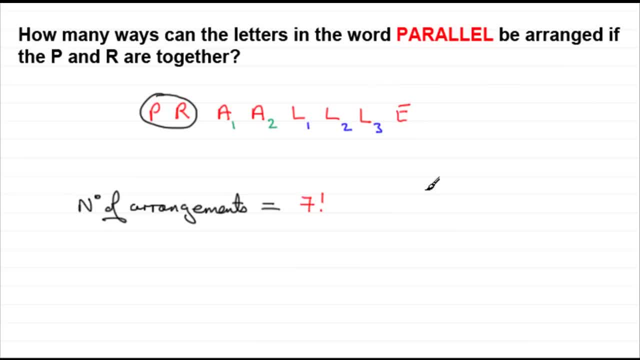 an R and a P, But what we'll just do is we'll write down that it's times two factorial. Now the point is that for any of these arrangements- remember we're treating these as if the A's and the L's are different, but they're not. If these subscripts were taken away for the